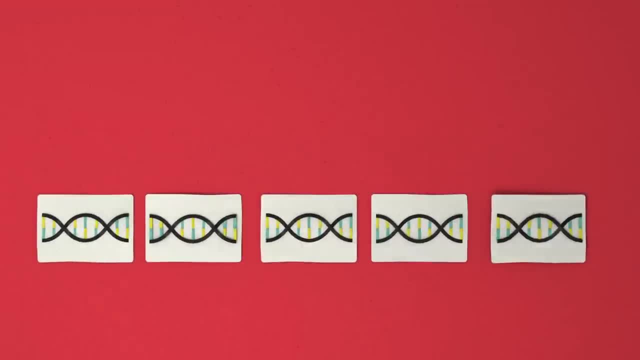 The first are short snippets of repetitive DNA sequences called Clustered, Regularly Interspaced Short Palindromic Sequences. Clustered Regularly Interspaced Short Palindromic Sequences, Or simply CRISPRs. The second are Cas, or CRISPR-associated proteins. 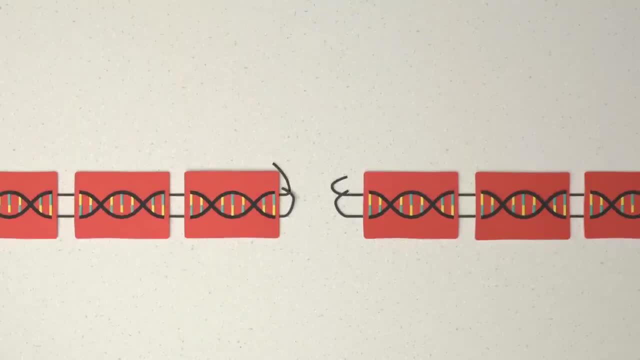 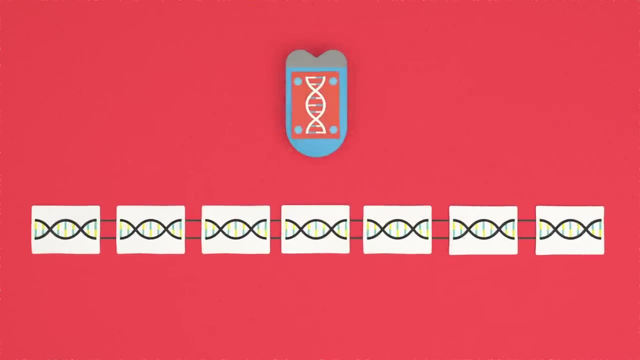 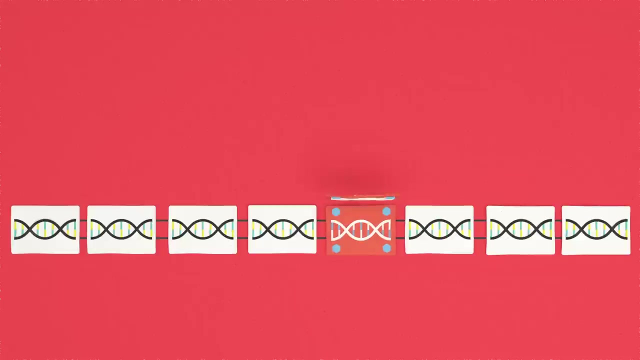 which chop up DNA like molecular scissors. When a virus invades a bacterium, Cas proteins cut out a segment of the viral DNA to stitch into the bacterium's CRISPR region, capturing a chemical snapshot of the infection. Those viral codes are then copied into short pieces of RNA. 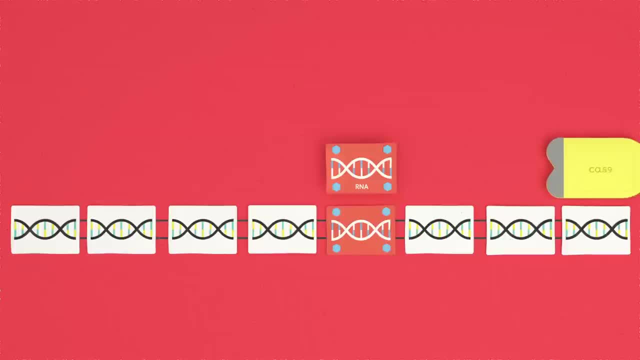 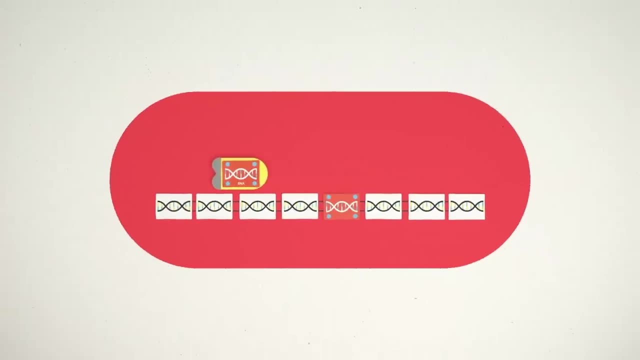 This molecule plays many roles in our cells, but in the case of CRISPR, RNA binds to a special protein called Cas9. The resulting complexes act like scouts, latching onto free-floating genetic material and searching for a match to the virus. 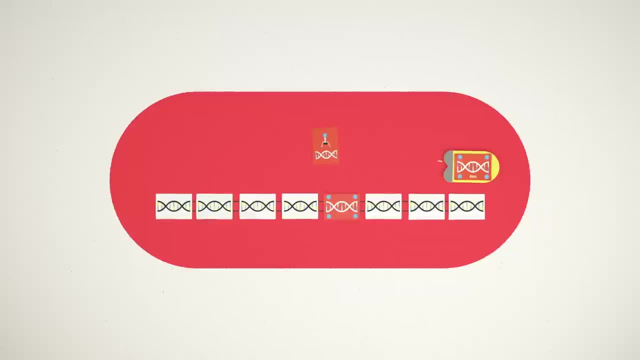 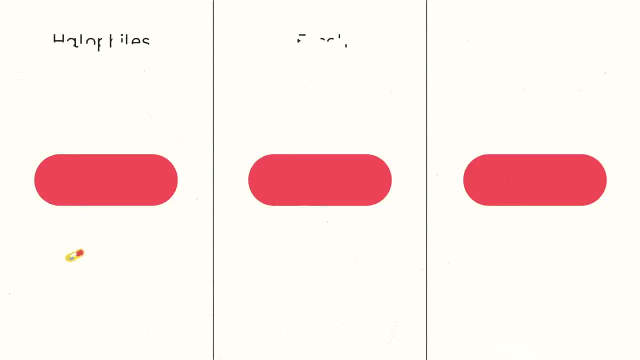 If the virus invades again, the scout complex recognizes it immediately and Cas9 swiftly destroys the viral DNA. Lots of bacteria have this type of defense mechanism, but in 2012,, scientists figured out how to hijack CRISPR to target not just viral DNA. 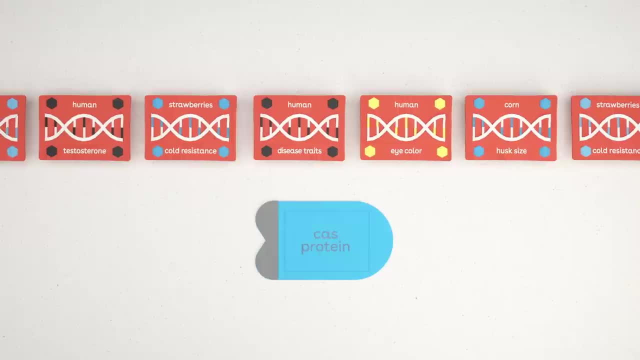 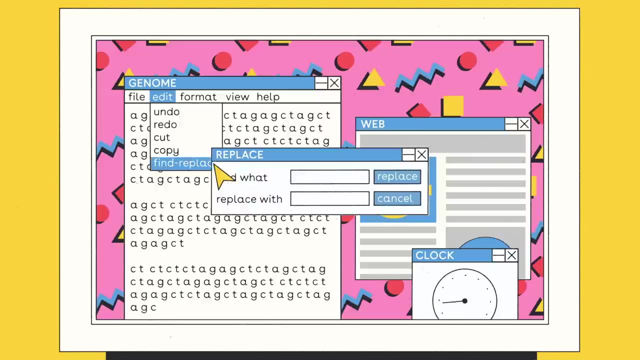 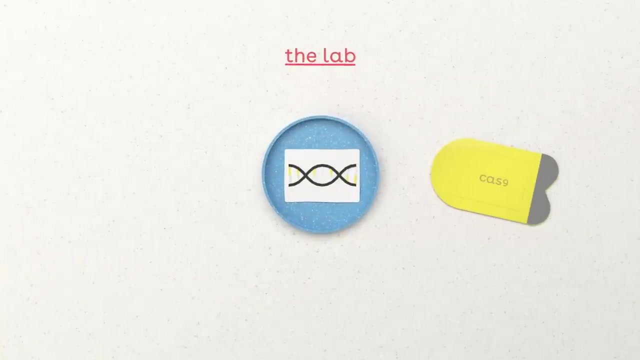 but any DNA in almost any organism. With the right tools, this viral immune system becomes a precise gene-editing tool which can alter DNA and change specific genes almost as easily as fixing a typo. Here's how it works in the lab. Scientists design a guide RNA. 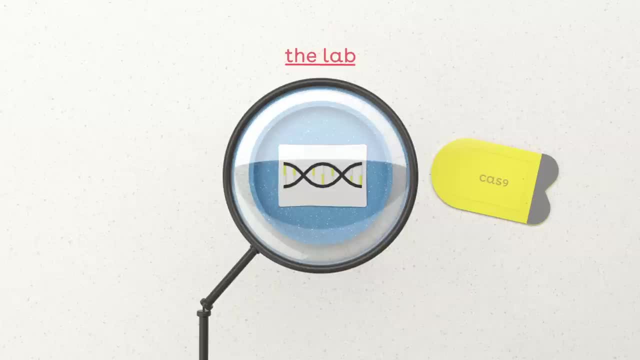 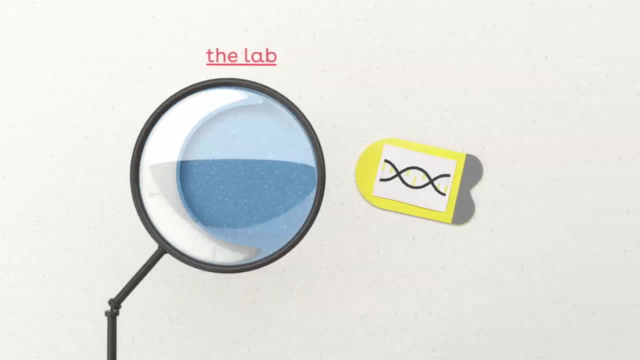 to match the gene they want to enter. First, they edit and attach it to Cas9.. Like the viral RNA in the CRISPR immune system, the guide RNA directs Cas9 to the target gene and the protein's molecular scissors snip the DNA. 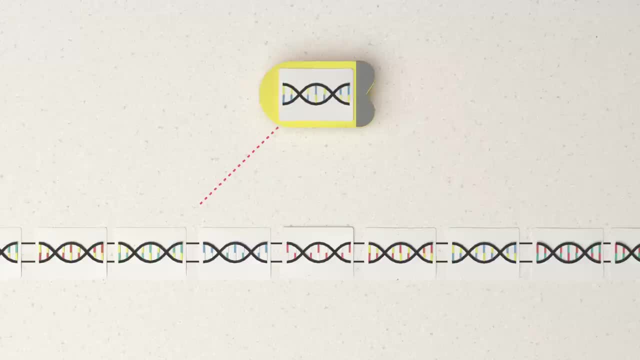 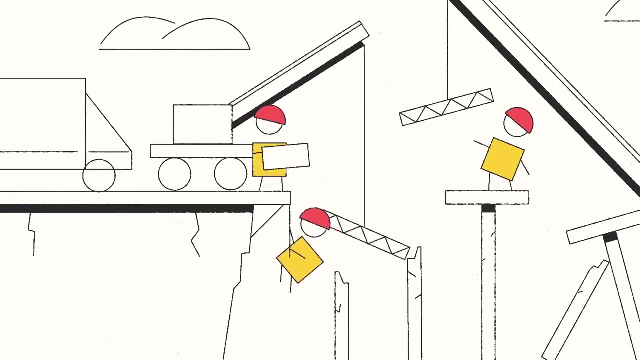 This is the key to CRISPR's power. Just by injecting Cas9, bound to a short piece of custom guide RNA, scientists can edit practically any gene in the genome. Once the DNA is cut, the cell will try to repair it, Typically proteins called nucleuses.